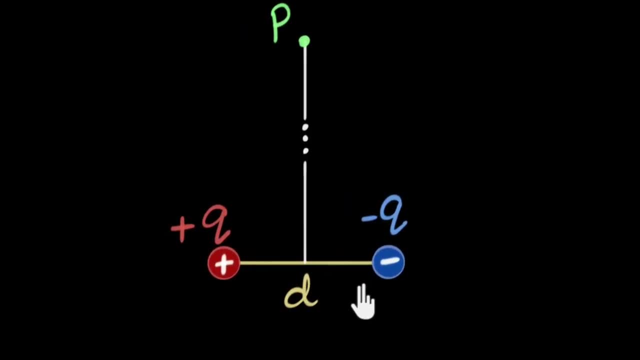 am, let's begin. So here we are. we've zoomed back in- And this is the point- very far away from the dipole, And that distance is r. Now again we could ask where? what? what distance exactly is r? Should I consider r to be from the point? 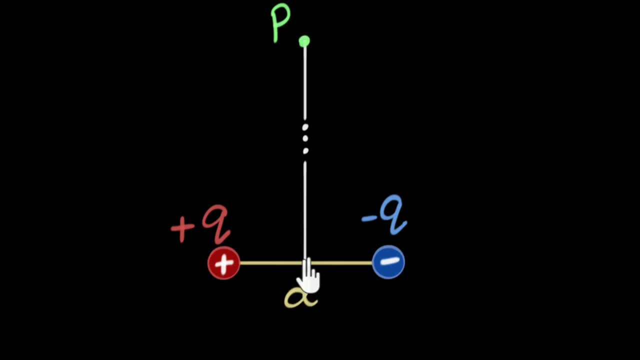 p to the center of the dipole. Well, that's what your textbooks do, And I think that's the safe way of doing this, But, just like in our previous video, we can be a little bit more adventurous. Remember, if I zoom out, the dipole looks like a dot, And so, whether you consider that, 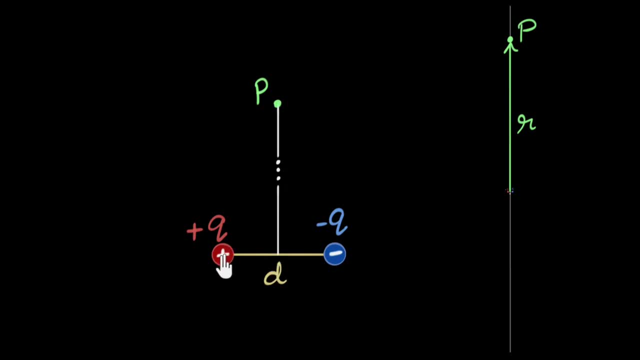 distance from here to here, or the distance from here to here, or from here to here. they're going to be exactly the same. So what we're going to do is we're going to zoom out and we're going to take the distance from here to here, or the distance from here to here, or from here to here. 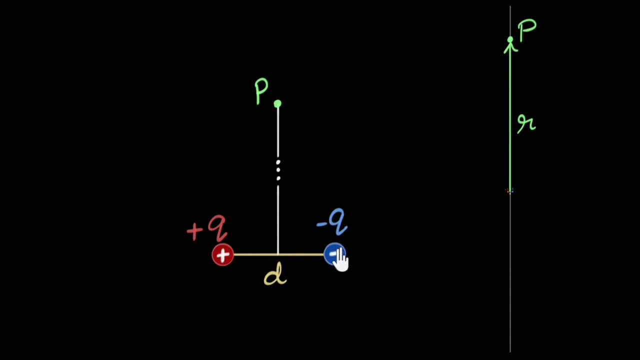 all should be pretty much the same. we can say they're all- almost all- equal to r, So I can say this is r, or I can also say this is r, And so what I'll do is: and what we'll do is we'll be a little. 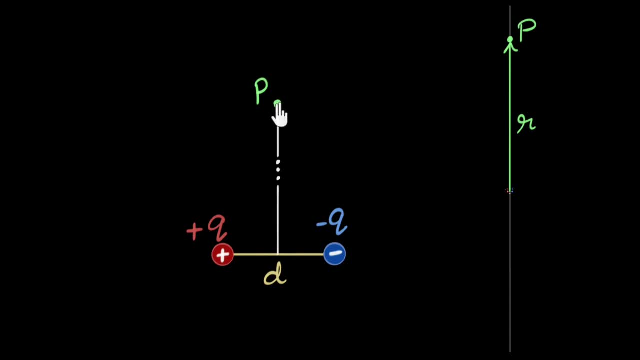 bit adventurous. we'll deviate from the textbook a little bit. we'll get the same answer should, and we'll call this distance as r. The expression will become just a little simpler. That's it, no other reason, And it's always fun to try to do things a little differently. 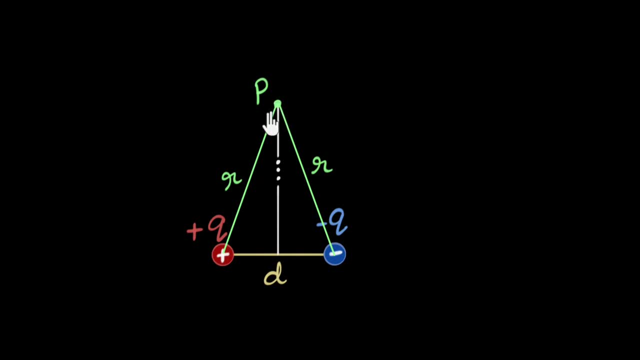 Alright. so how do we begin? Well, I need to find the electric field here and I can use my superposition principle, which says the field here is going to be feel due to this charge alone, plus do feel due to the discharge alone over here. So why don't you pause the video and think about? 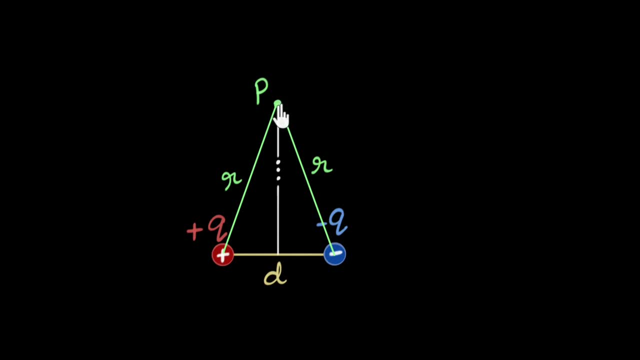 what the individual fields are going to be due to the plus q and minus q And also see if you're going to write the direction of those individual fields, draw the direction of the individual fields. Can you pause and try that yourself first? Okay, so due to the positive charge, 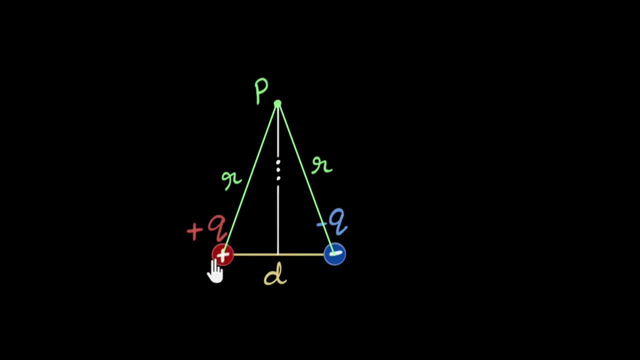 electric fields always away from the positive charge. So we're here. electric field will be away from it and along this line away. So the field would look somewhat like this And if I consider the negative charge, field is towards it, again along the line joining. so the field will be. 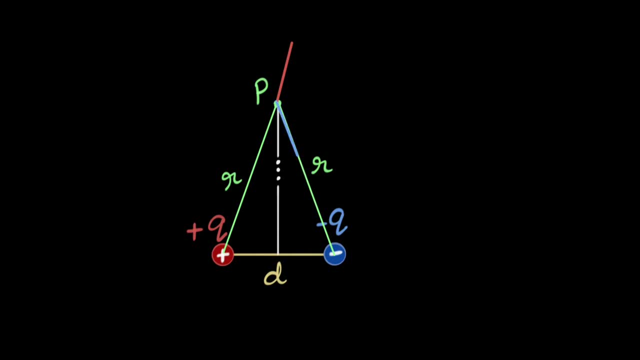 somewhat like this: Let's draw the arrow marks: This is our electric field due to the negative charge, And this will be the electric field due to the positive charge. Alright, now we need to add these two vectors up and they're not in one dimension. we need to be a little bit careful. 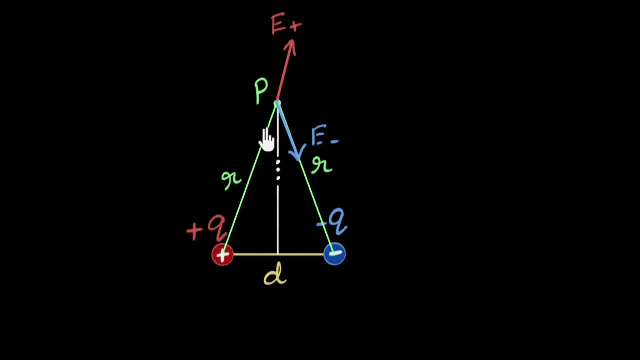 So the first thing is: let's look at the magnitudes. Well notice: the charge is the same, magnitude of charge is the same and the distance is also the same. So the magnitude of the electric fields must be the same, right? Because it's k times q divided by r square. So we can immediately say hey, 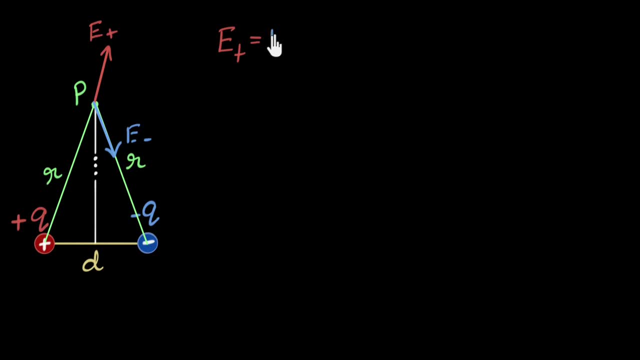 the electric field due to the positive charge should equal in magnitude the electric field due to the negative charge, And that equals k, which is the Coulomb's constant one by four pi, epsilon naught, nine times 10, to the power, nine times q, the charge is the same. This is the 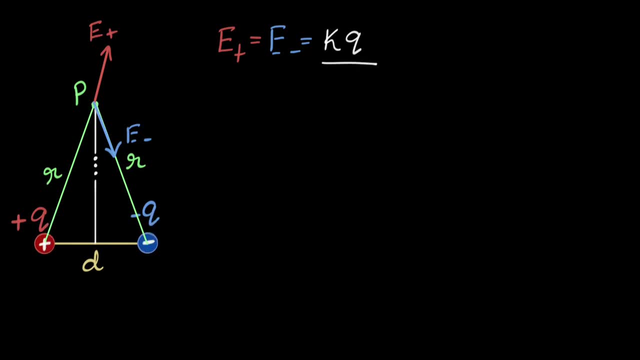 magnitude I'm looking at divided by the distance squared. and the distance is the same, r. So it's going to be divided by r square. So we now have two equal vectors and we need to figure out what the resultant is going to be. Hmm, how do we do that? The physics is pretty much done now. it's a. 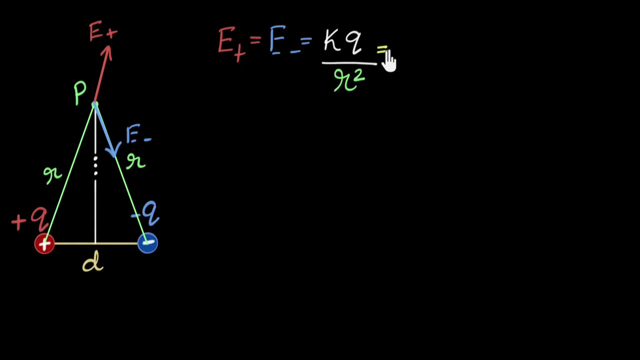 math problem. So the first thing we can do is, because the two vectors are exactly equal in magnitude, let's just give it one name, Let's just call it E. So this will be E and this vector will also have the same magnitude, E. Now how do we look at, how do we calculate the 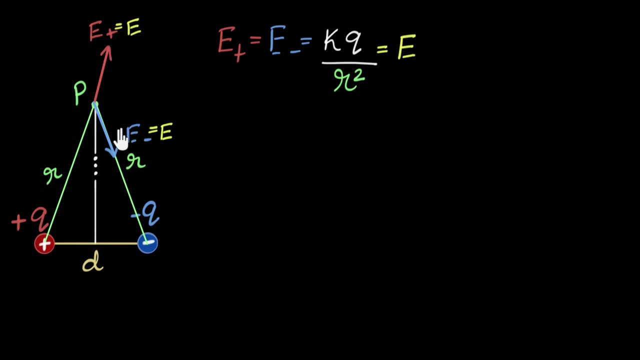 resultant. One way is to use the parallelogram or the triangle of vector addition. Another way is to decompose the vectors and use perpendicular components, And I like that because it's more conceptual. Think of it this way. Imagine this: there is a ball over here and two people are. 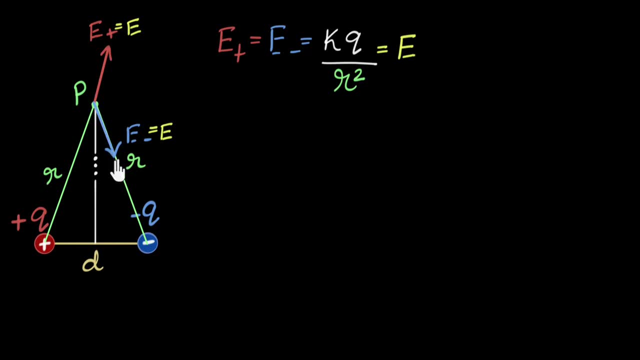 pulling it like this, with the same force. What direction would the ball accelerate? What? what is the net force it will experience? Well, because the two forces are exactly equal. there is no reason for the ball to accelerate towards any of these forces. So 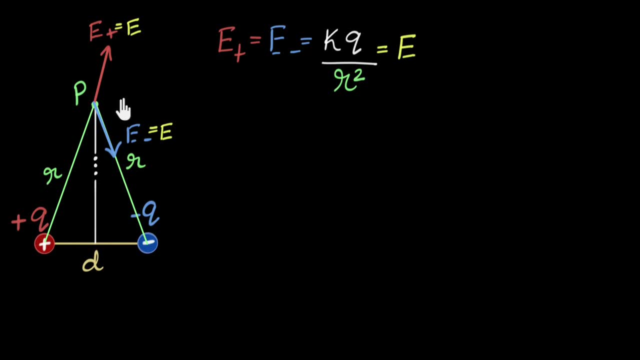 it will accelerate right in between them. And so we know for sure the resultant has to be right in between them. And so I can tell right from here: the resulting electric field has to be right in between the two, And from symmetry we could say the right in between has to be this way. 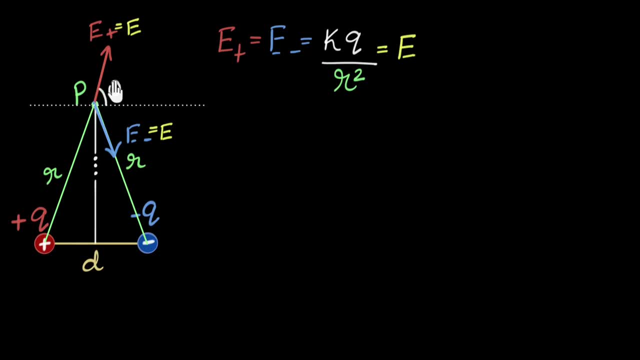 And so what we can now do is we can call this angle theta. This angle would also be theta, I'll just not write it, I don't want to, keep you know, make it too crowded. And then we can decompose each vector into this horizontal and vertical components, And we will see vertical. 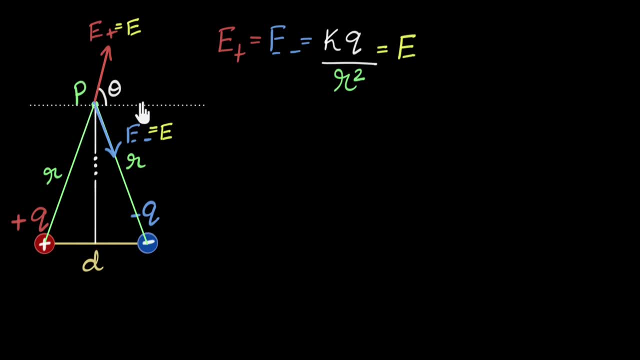 components subtract, they cancel each other, horizontal components add up And from that we can figure out what the net electric field is going to be. And to do this carefully, here is a zoomed in version of whatever I've drawn over here. I've drawn it better. 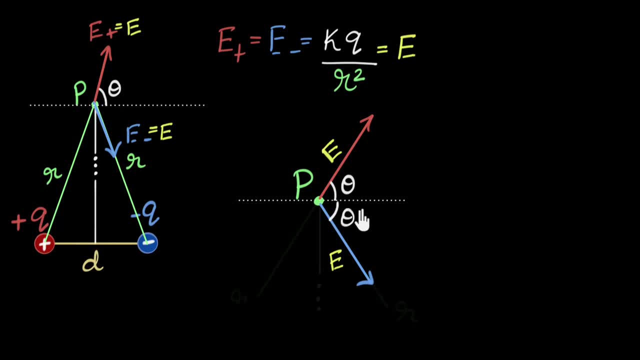 So why don't you pause the video and see if you can give it a shot? first, try figuring out what the net electric field is going to be by decomposing these vectors. So pause and try. Okay, let's start with this vector To decompose it, because I'm decomposing it into 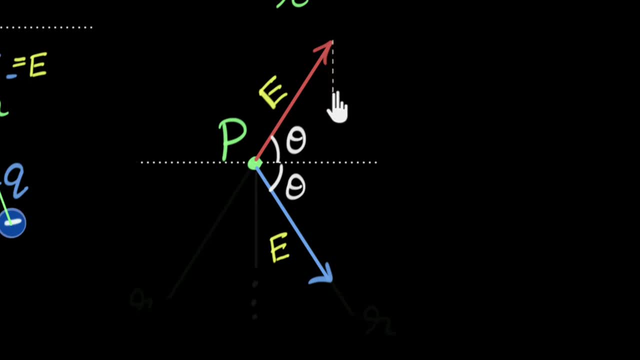 horizontal and vertical component. I'll just drop a vertical from here to here. And now I could say that, hey, this vector is the same as this vector. this is the horizontal component, plus this vector is the vertical component, And if this angle is theta, 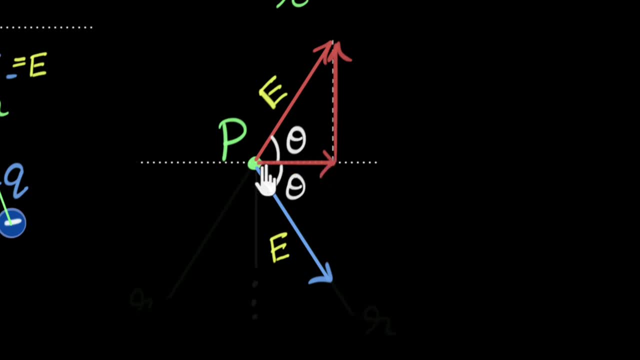 then this is the adjacent side. So if you use the trigonometry, you can say, hey, this is e cos theta. You can just, you can just confirm that this length will be cos theta. And what will this length be? Since this is the opposite side, this length will be e sine theta, And we can do the 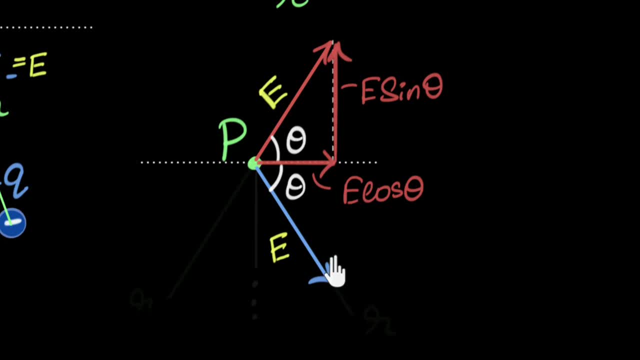 same thing with our blue vector. drop a perpendicular from here to here And we could now say there's going to be a horizontal component and a vertical component, And the horizontal component will be the exactly the same. it's going to be e, cos, theta And even the vertical component. 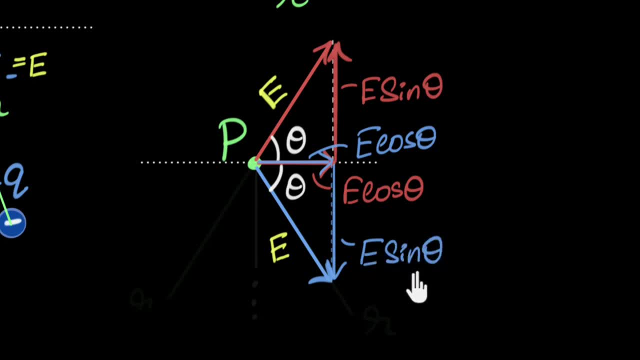 will be in magnitude exactly the same: e sin theta. And now look at what happens. The vertical components are exactly equal and opposite. They cancel out. So what remains is the horizontal component. they add up. so I get to e cos theta Again. it's got a little crowded over here, But 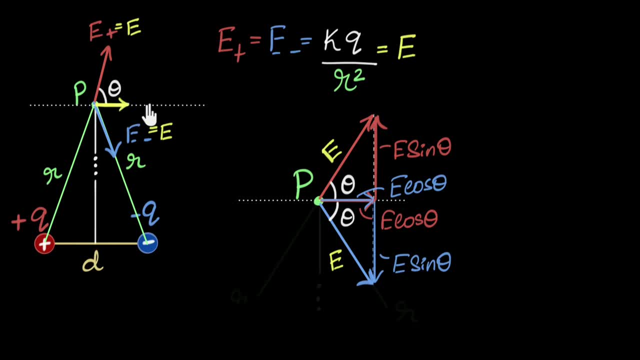 now I can finally write. So I know my net electric field over here is going to be 2e cos theta, So let's write that. So net electric field is going to be 2e cos theta When I write the vector. there's 2 e cos theta When I write the resulting healing part of e cos theta. So let's make myiyet that so e cos theta. So that's why I write watts each and also numbers per second. I'll make my estiver for e cos theta. 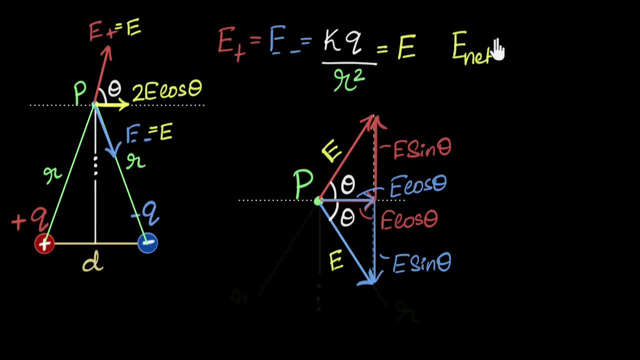 All right, I got a quick note. I know that so nowadays when I apply the other terms in the text too, but now that happens in the text, write that. so net electric field on the equator is going to be 2. i know the value of e is the. 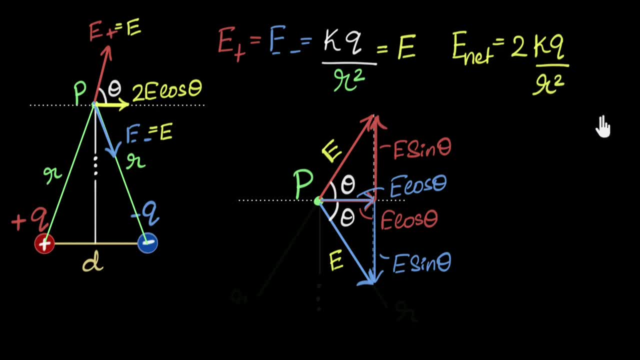 field due to individual charges. k into q, divided by r, squared times cos theta. now the only thing i need to figure out is what cos theta is. how do we do that? but can i use these, these triangles, and use trigonometry? no, because i used angle theta to figure out what the side lengths are. i didn't. 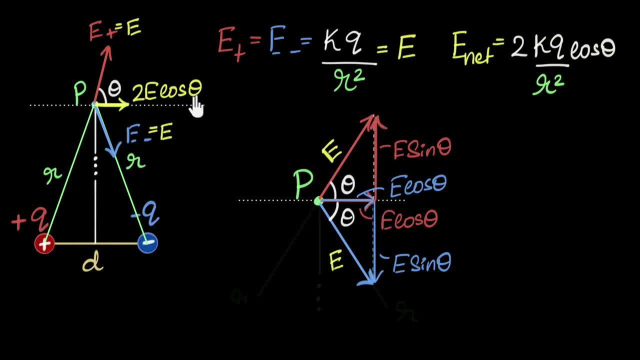 know the side lengths to begin with. so the question is: how do i figure out cos theta? i can use a little bit of geometry and there's a triangle right over here, so maybe i can figure out, okay, if this angle is theta in this triangle, where theta is going to be, and then i can use the sides of. 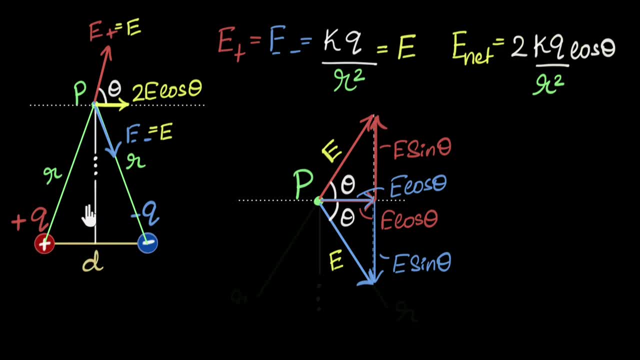 that triangle to figure out cos theta. so it's the last part. and again, if you, if you couldn't do it before, no worries, last part. can you pause and see if you can complete this? all right, let's bring this home. so if this angle is theta, then this angle is a corresponding angle to it, because 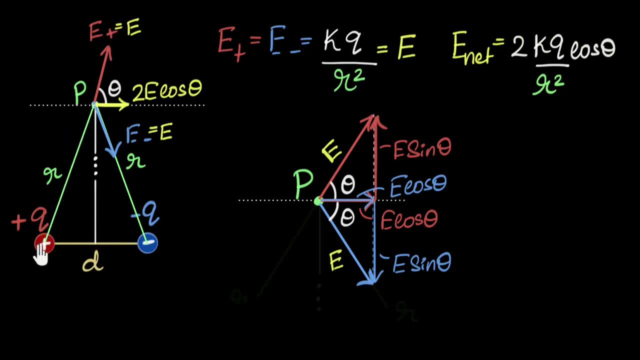 this is a parallel line, so this is a straight line and you have these two parallel lines. so this angle is theta, and so i can from this triangle- cos theta is the adjacent side divided by the hypotenuse- i can write that. so let's do that. so the net electric field is going to be: 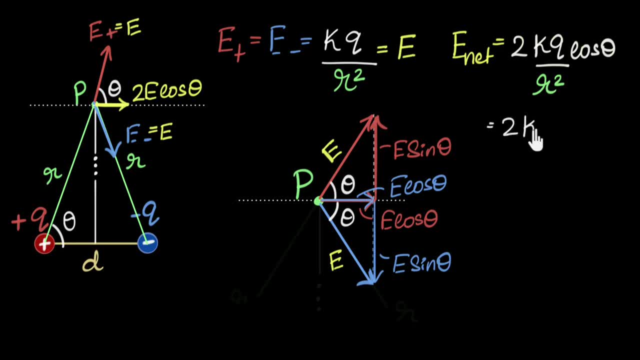 let me just write this: equals 2kq divided by r, squared times cos theta, which is the adjacent side. what is this? well, the whole distance is d. well, this is half of d. so it's going to be d over two adjacent side divided by the hypotenuse r. and guess what we have gotten it? we found the. 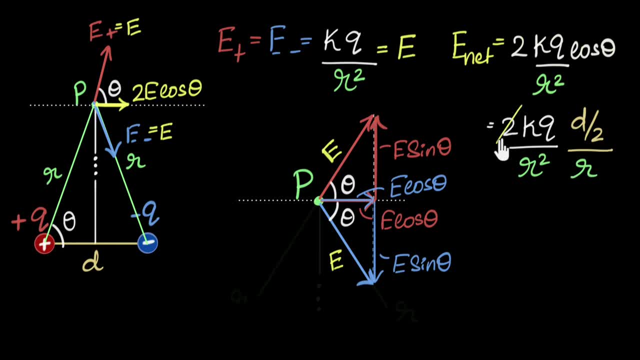 answer: we have everything, and so let's put it all together. so two cancels out, and so what i'll end up with is k into q into d, divided by r cubed, and so the net electric field is going to be the coulomb's constant k q times d. hey, what is q times d? i think you know this. 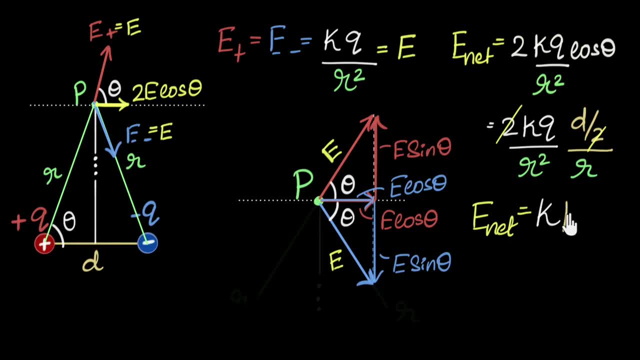 q times. d is a dipole moment. we've introduced this before in previous videos and i'm pretty sure now you're familiar with this. divided by r cubed, divided by r cubed, and i think we should box this. this is the fruits of our hard work. 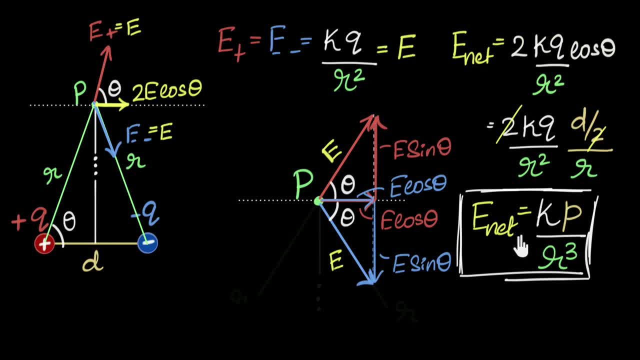 the last thing about this expression is: what is what about the direction? well, over here the direction is to the right. but let's compare it with respect to the dipole moment. what direction is the dipole moment? for a given dipole, it's always from negative to positive charge this way. 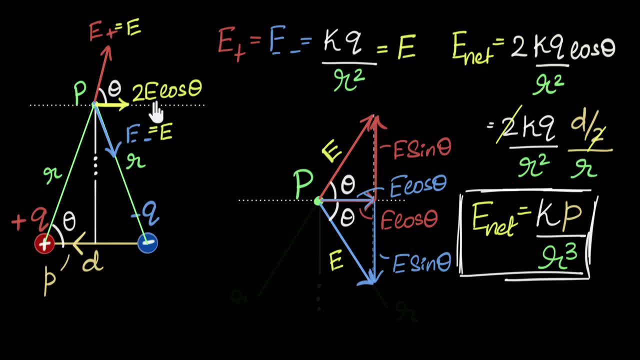 this is the direction of the dipole moment and therefore you can see on the equator, the electric field is in the opposite direction of the dipole moment and that's why we often write vectorially: this is on the equator minus when you write it in vector form, because it's in the opposite direction of the dipole moment. 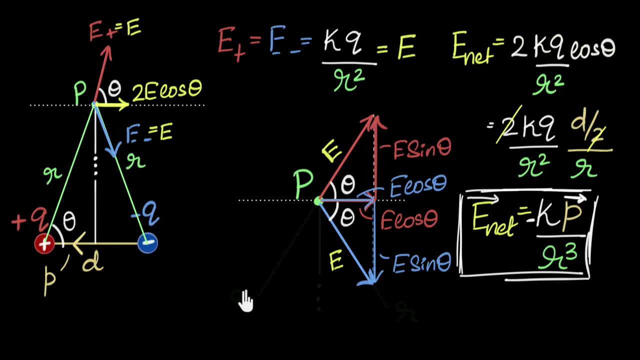 i'm going to take the last couple of minutes to digest this and make sense of dipole in general. so first thing i want to do is compare this with the electric field that we got on the axis. if you remember that, you'll find on the axis electric field is very similar but two differences. 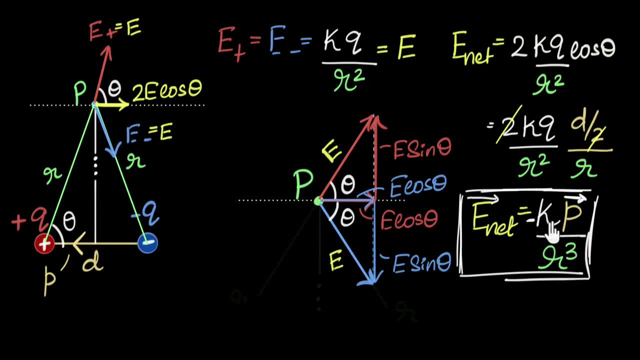 it was 2 kp by r cube, so twice the magnitude. and the second is on the axis. the electric field was in the same direction as the dipole moment and i want to try and understand that. why has the strength become half and why has the? you know why is it is in the opposite direction. for that 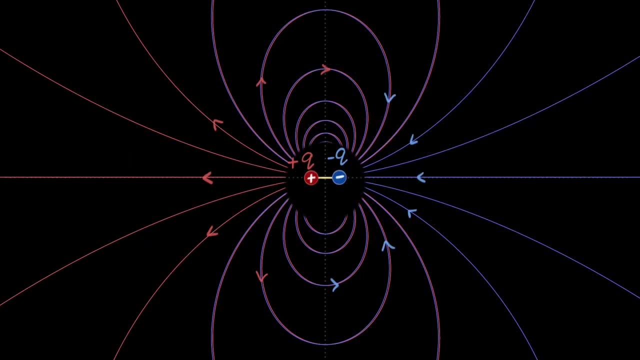 we can zoom out and re-look at the electric field lines. first let's think about the strength. see from an electric field lines point of view. the field lines are closer, the strength is more, and if the field lines are farther away, the the strength is weaker. so if you take any two field lines, let's 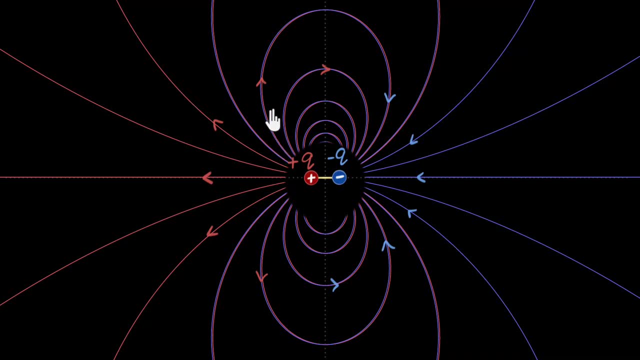 say you take these two or maybe these two field lines, you can see as they come towards the axis, that's where they are the closest. and as you go away from the axis, near the equator, notice the field lines are the farthest apart. then again they become closer to each other. so just from the field,